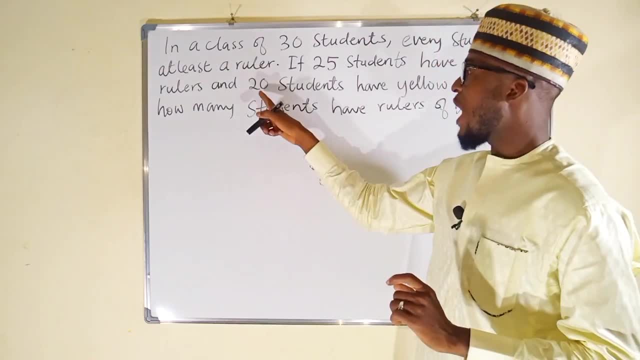 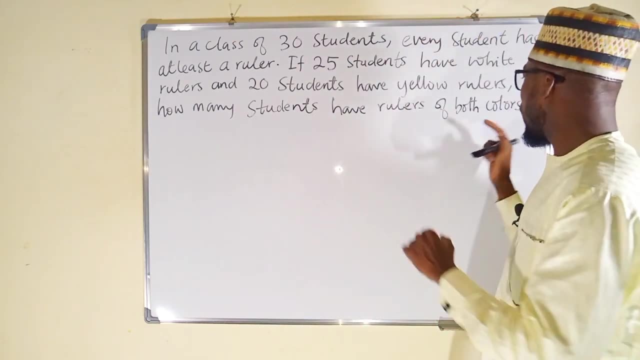 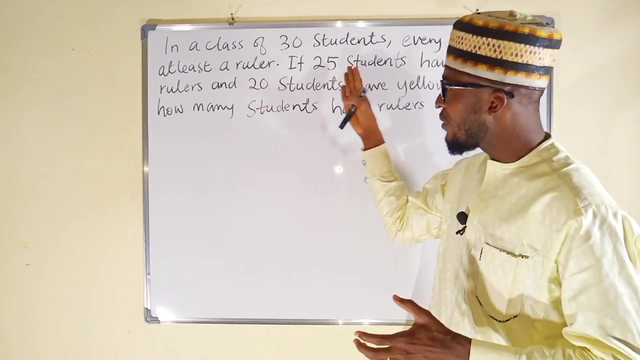 rulers. Take note of that. And 20 students have yellow rulers. How many students have rulers of both colors? Let us understand this question, because you have to be able to interpret these words into mathematical statement. In a class of 30 students, it means a. 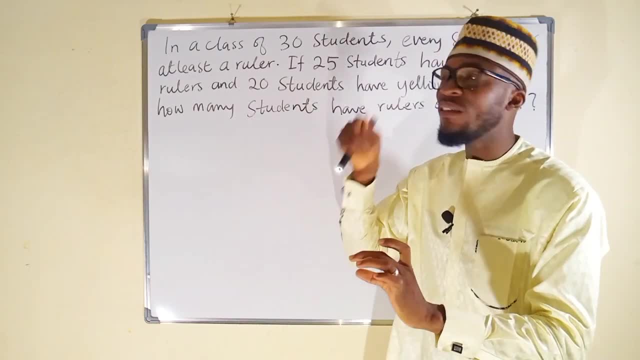 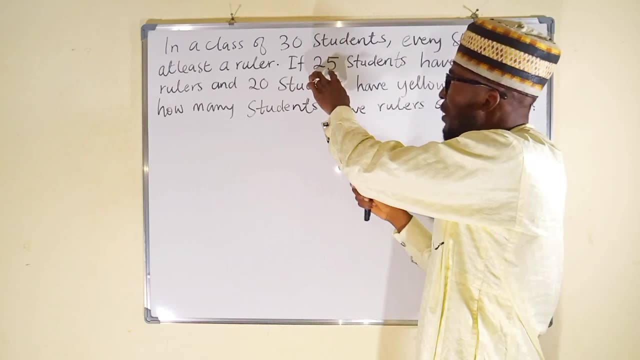 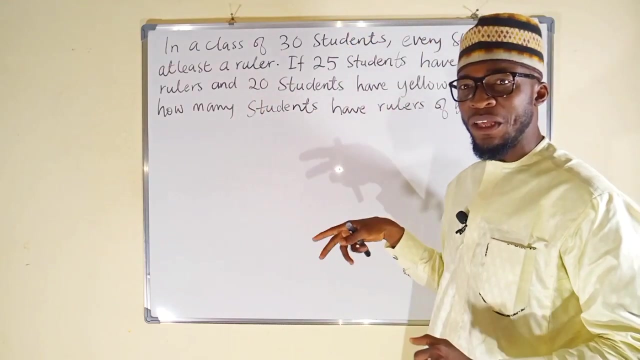 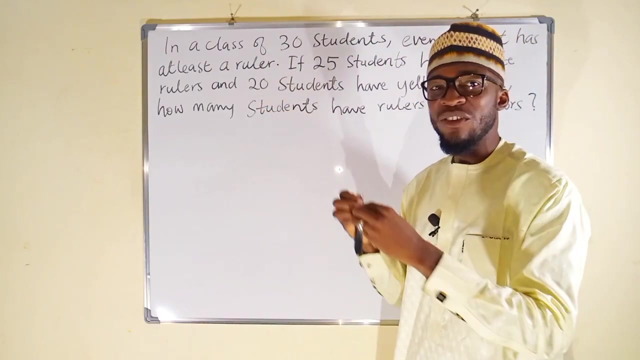 particular class that contains only 30 students. We have two groups. The first group of students- there are 25 that have white rulers and 20 of them have yellow rulers. You can see the combination exceeds the number of students in the class. why this is 25. this is 20 joined together. we 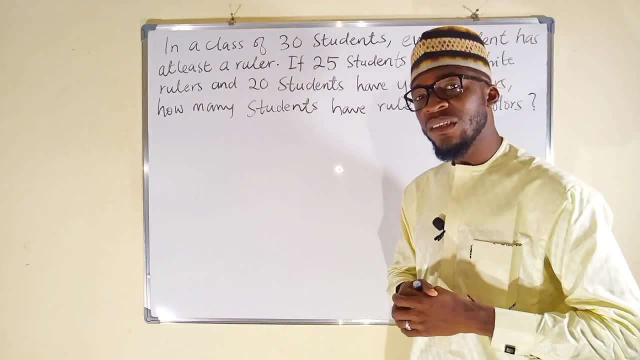 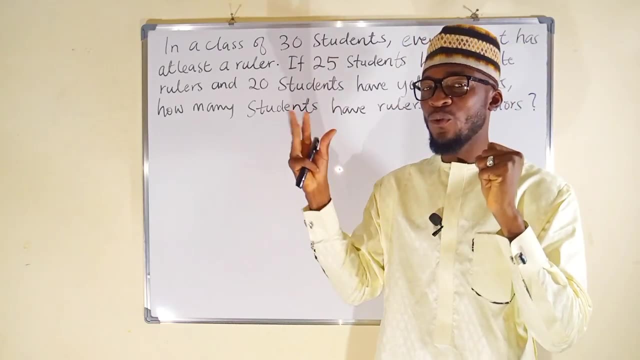 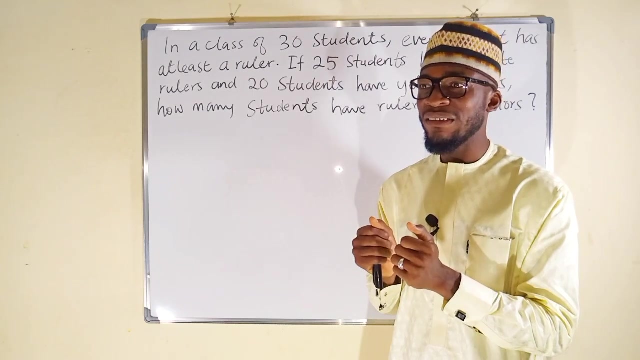 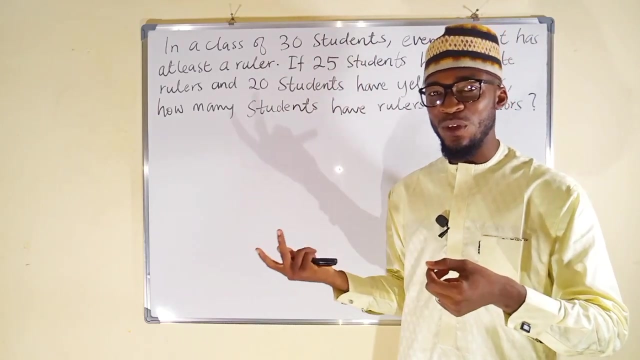 have 45, but this is 30. the reason is that there are some students among these 30 students that have yellow rulers as well as whites rulers in their position, so they are going to be categorized at the middle. that is, the intersection between the two sets, because we have two sets here, white and yellow. so those that 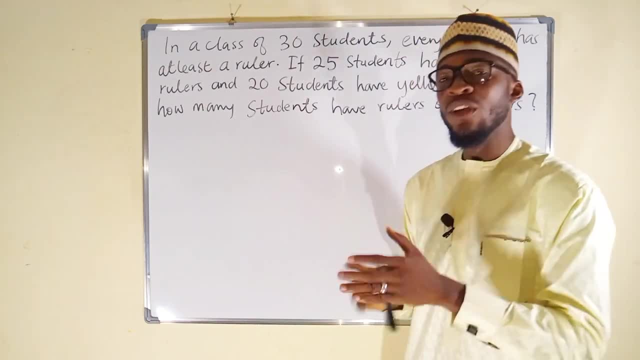 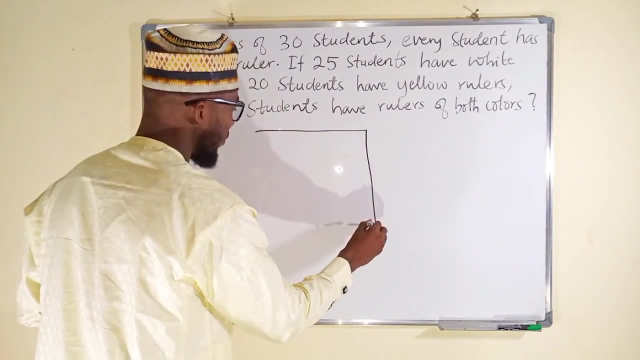 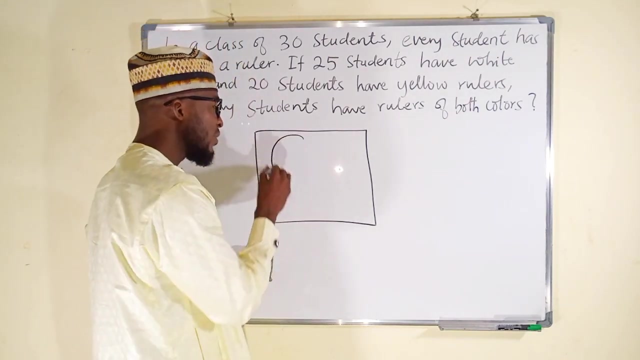 have white and yellow should come to the center, their intersection. so let me use a Venn diagram to explain this properly. I don't have to talk about the theoretical aspect of Venn diagram, because I have discussed about it in some of our previous lessons. we have only two sets, and these two sets 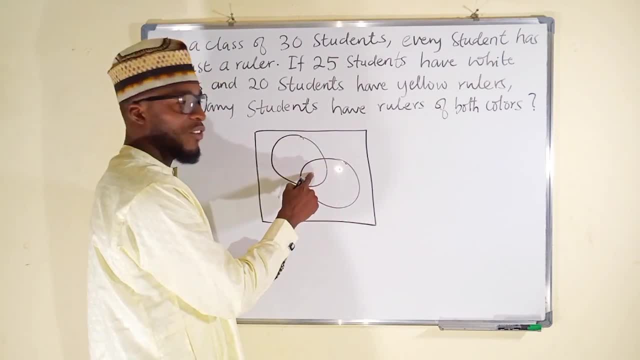 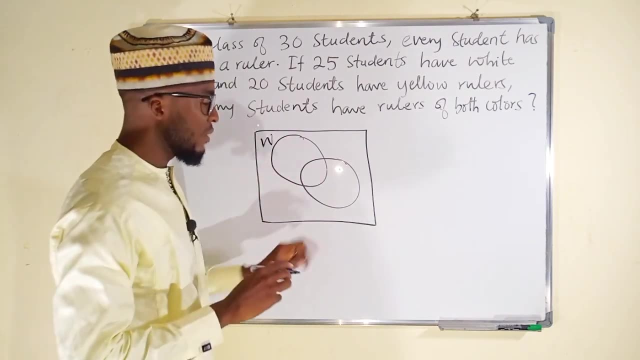 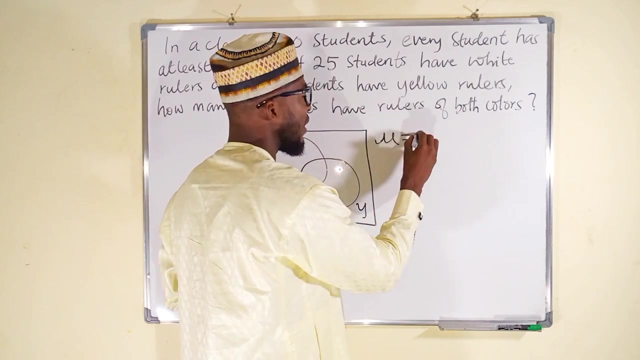 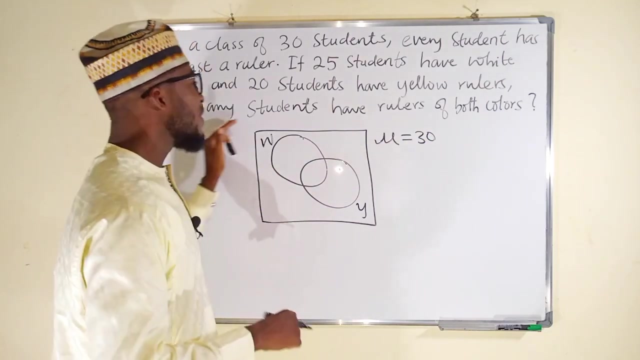 intersect. this is the intersection, so let this set. this cycle represents the number of students that have white rulers, and this should be yellow, and the universal set, which is the total number of students. they are just 30, so if you add everything in this set, you must obtain 30. this question is: 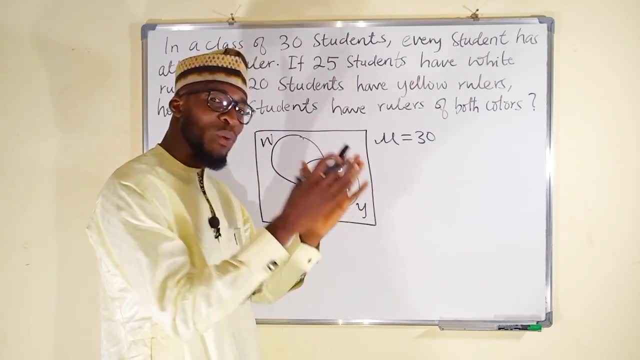 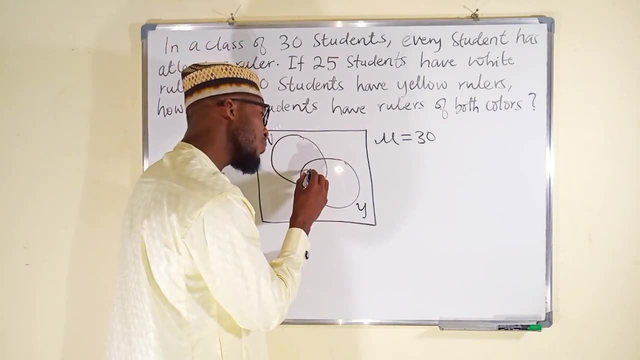 asking us to find the number of students that have white rulers as well as yellow rulers, and they are said to be the intersection between the two sets, and we don't know them. we can call them X. this center is said to be the intersection between the two sets, so 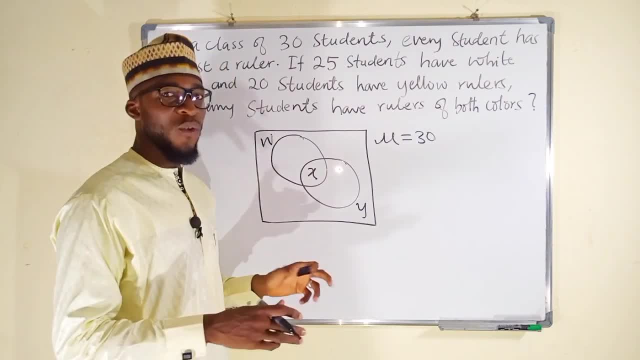 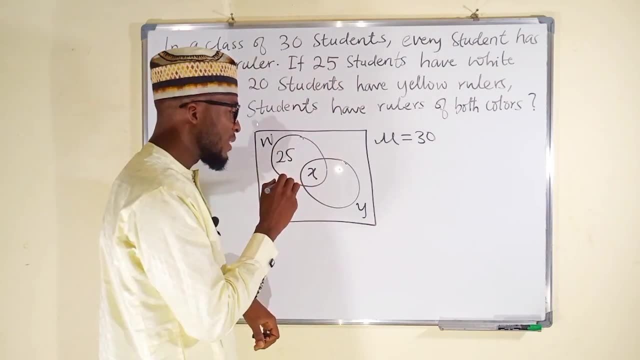 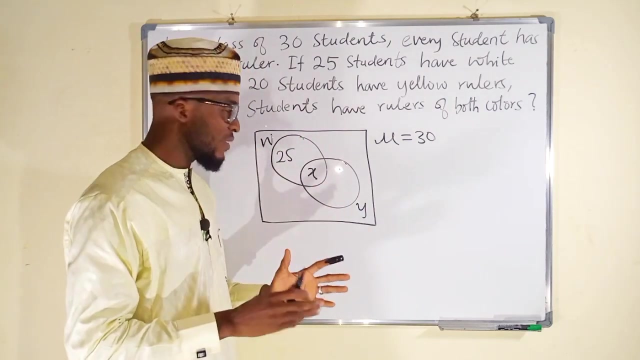 let's start with white rulers. the number of students that have white rulers: they are 25, but we are not going to write 25 here, because this is also part of 25. you can see the whole cycle. the whole of this cycle contains 25 students, but these 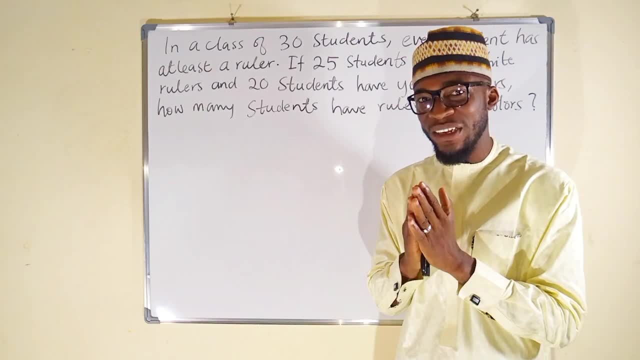 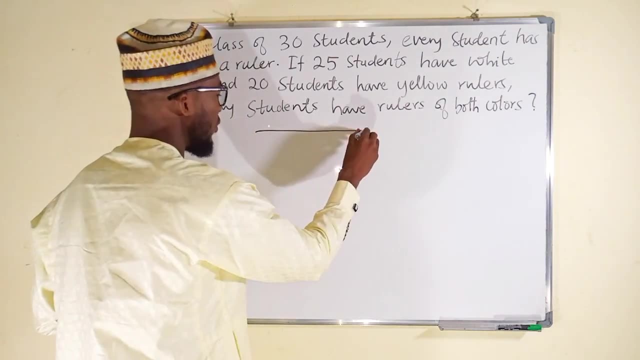 So those that have white and yellow should come to the center. They are intersection, So let me use a Venn diagram to explain this properly. I don't have to talk about the theoretical aspect of Venn diagram, because I have discussed about it in some of our 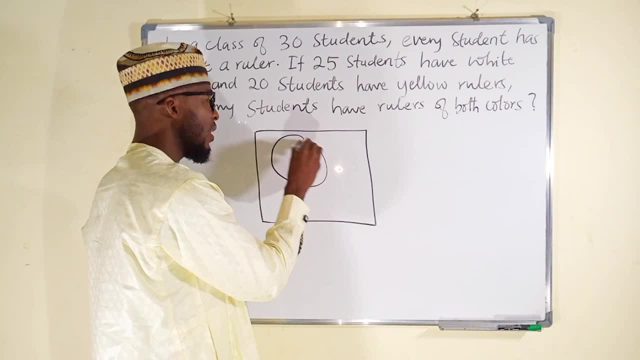 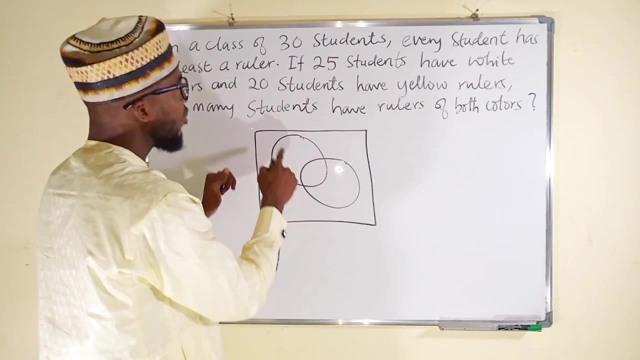 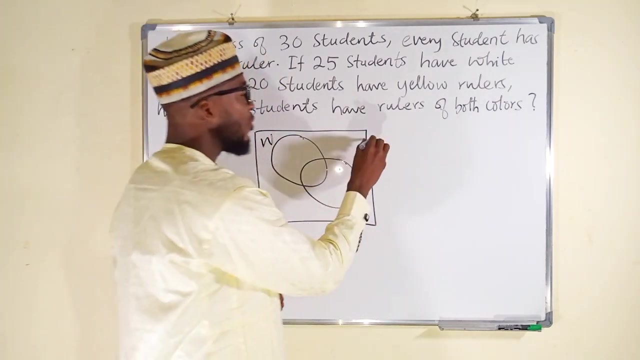 previous lessons. We have only two sets and these two sets intersect. This is the intersection, So let this set, this cycle, represent the number of students that have white rulers, And this should be yellow, And the universal set, which is the total number of students. 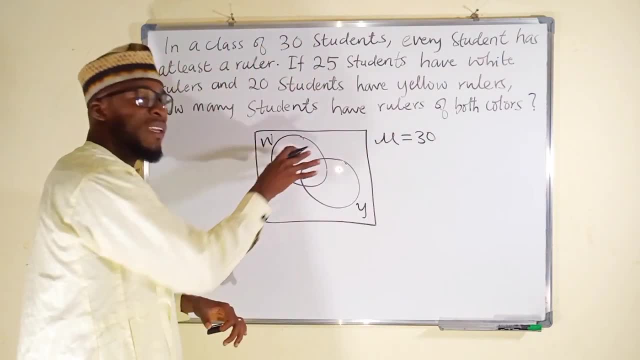 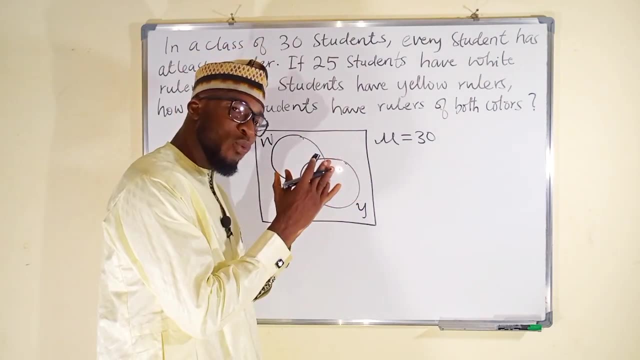 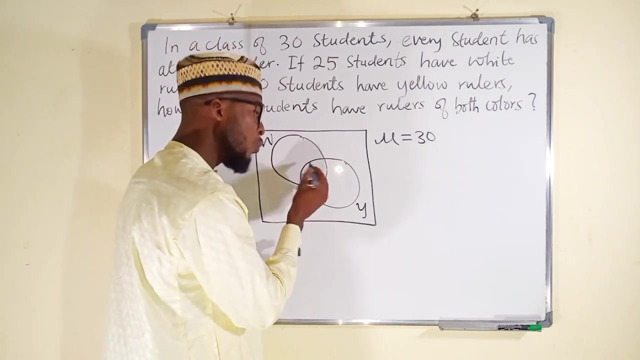 they are just 30. So if you add everything in this set, you must obtain 30. This question is asking us to find the number of students that have white rulers as well as yellow rulers, And they are said to be the intersection between the two sets, And 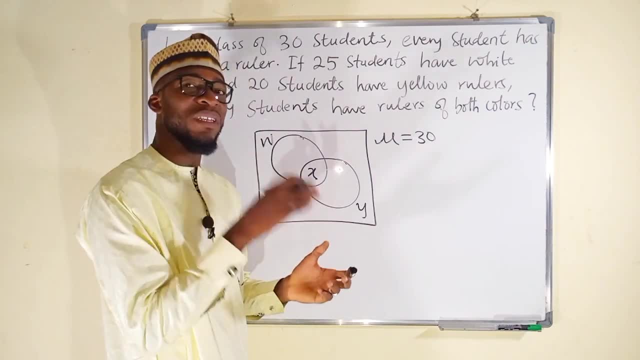 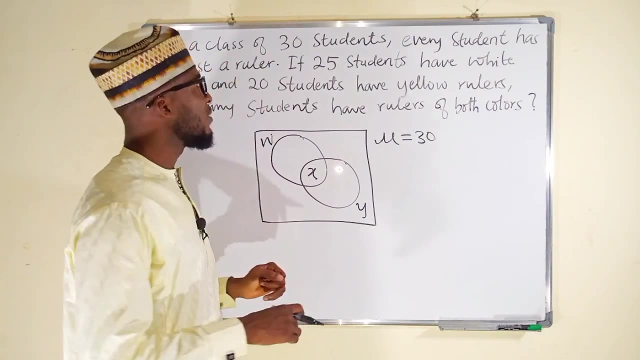 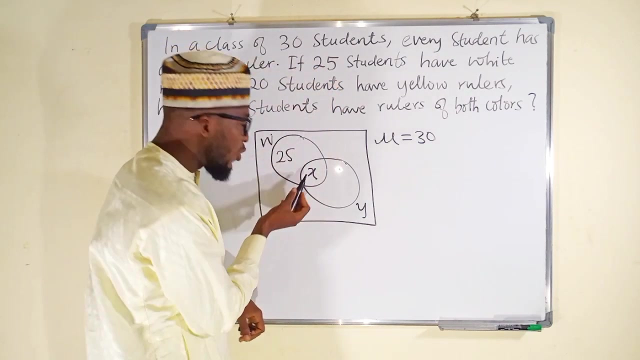 we don't know them. we can call them X. This center is said to be the intersection between the two sets. So let's start with white rulers. The number of students that have white rulers: They are 25.. But we are not going to write 25 here, Because this is also part of 25.. 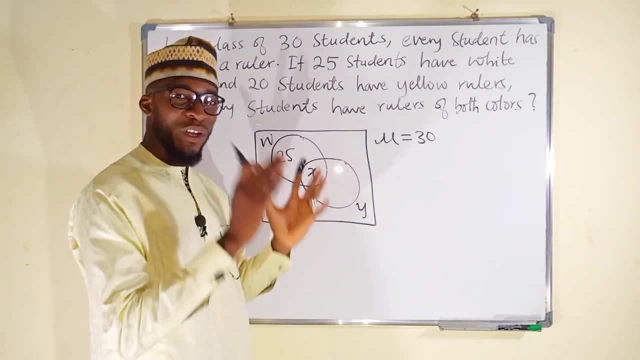 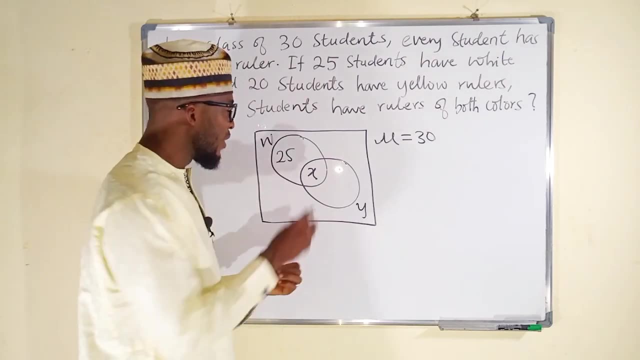 You can see the whole cycle. the whole of this cycle contains 25 students, But these people here that we are looking for, they have both white and yellow rulers, So we have to subtract X here in order to find out only this portion here. 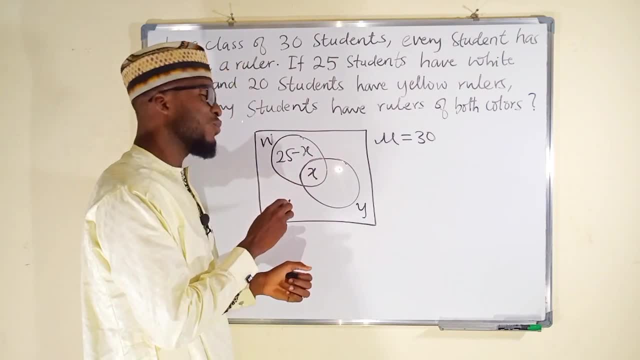 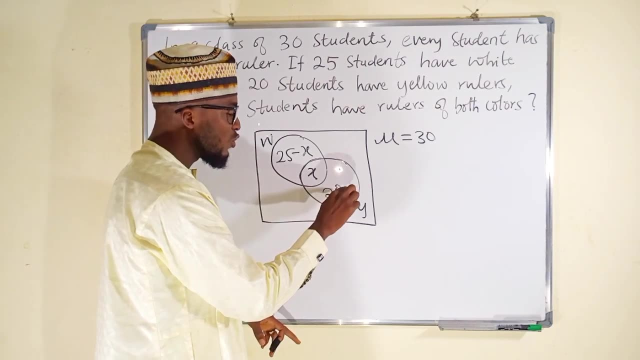 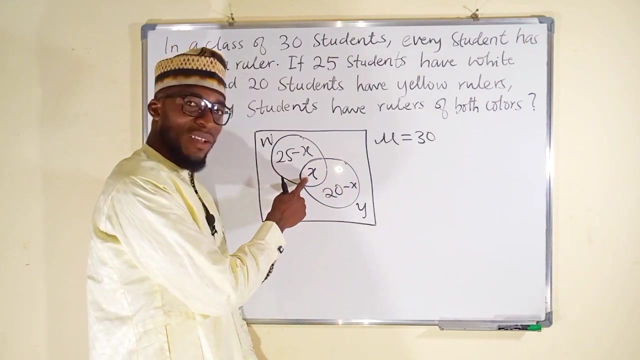 Only this portion without here. Only students that have white rulers should be here, And this one they are said to be 20.. And this 20 you have to subtract X from it, Because the whole of this cycle represent 25.. But we already have X here. So what is left here? 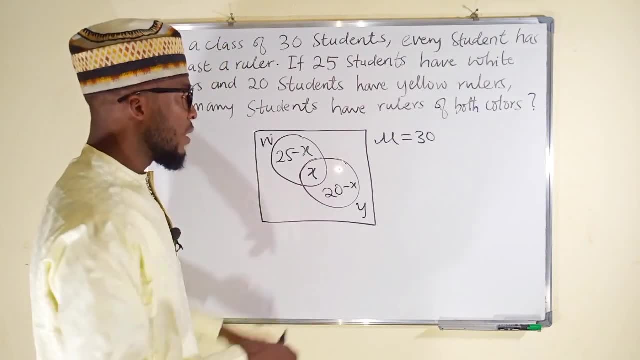 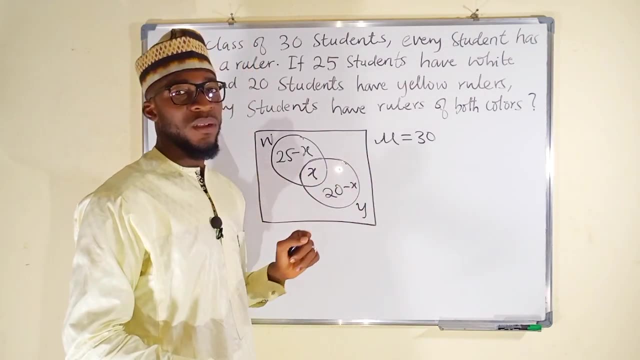 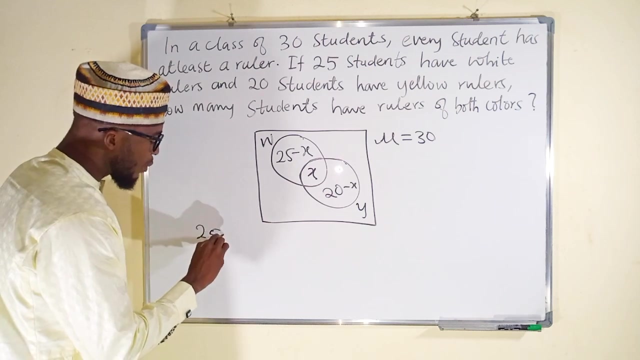 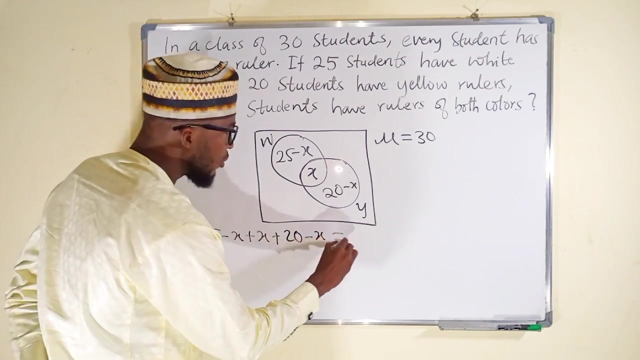 is going to be 20 minus X. If you add everything that you are seeing here, you must get 30.. Our main target is to find this value, This number of students, X, That X represents. So we have 25 minus X, This one Plus X again, Plus 20 minus X. We must get 30.. 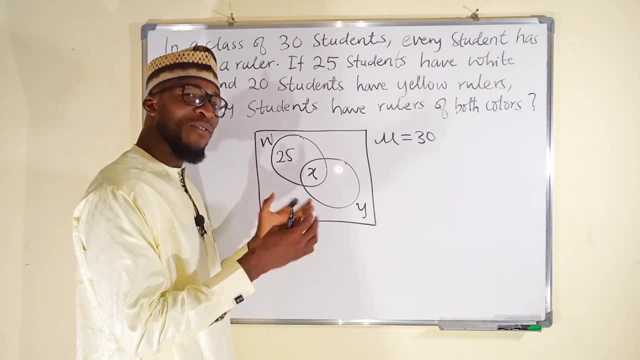 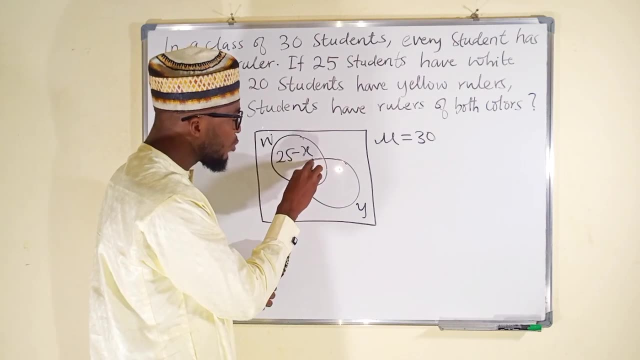 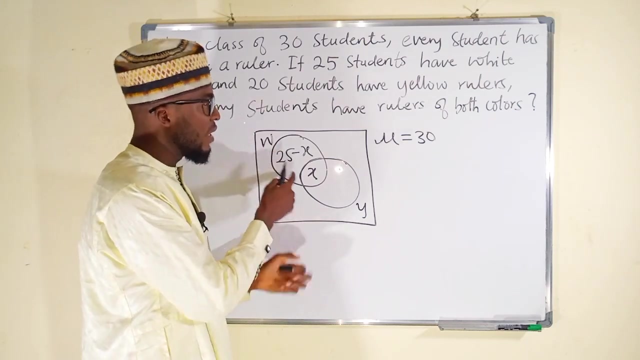 people here that we are looking for. they have both white and yellow rulers, so we have to subtract X here in order to find out only this portion here, only this portion without here. only students that have white rulers should be here, and this one they are said to be. 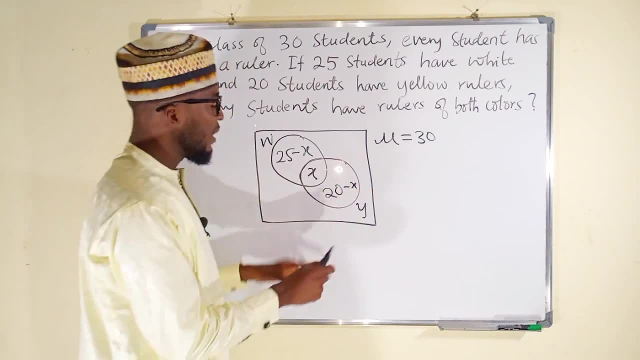 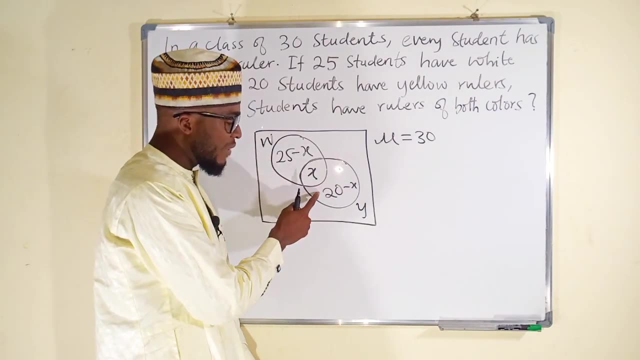 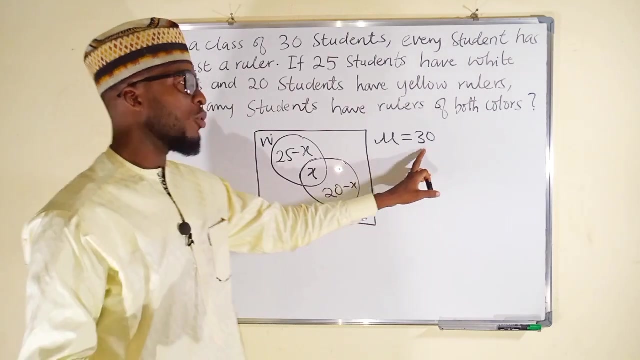 20 and this 20. you have to subtract X from it, because the whole of this cycle represent 25, but we already have X here, so what is left here is going to be 20 minus X. if you add everything that you are seeing here, you must get it. 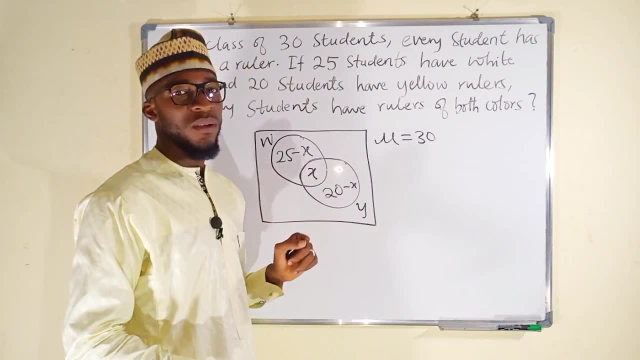 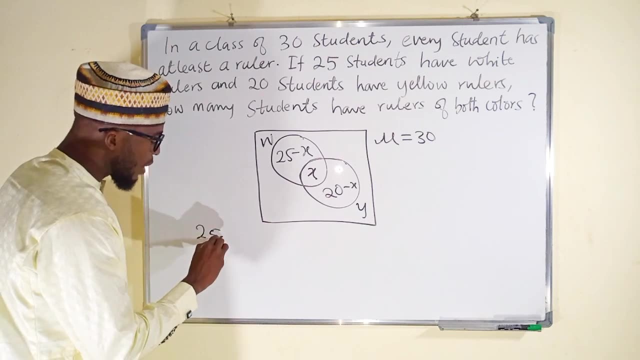 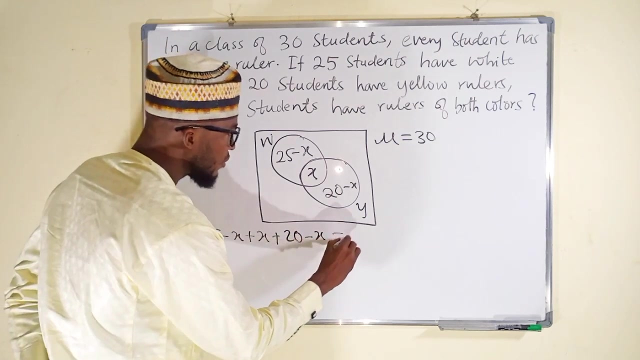 30. our main target is to find this value, this number of students, X, that X represents. so we have 25 minus X, this one plus plus X, again plus 20 minus X. we must get 30. this will cancel this, because this is negative. this is: 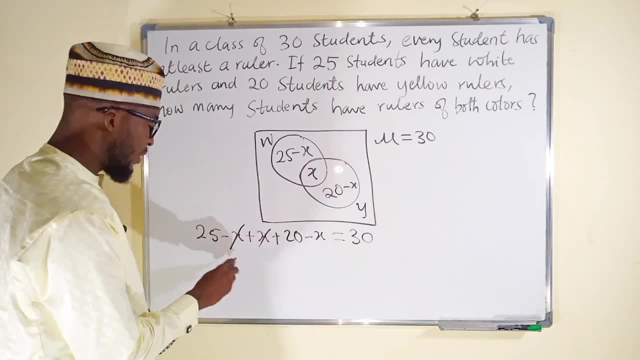 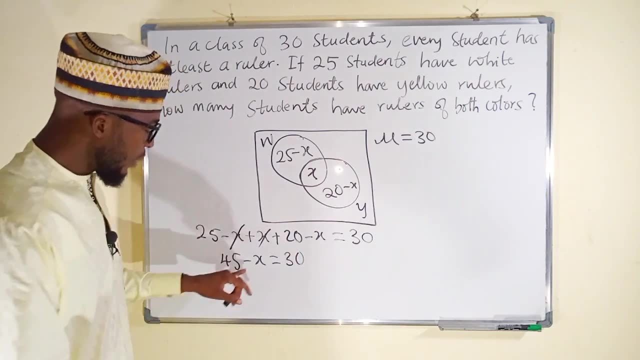 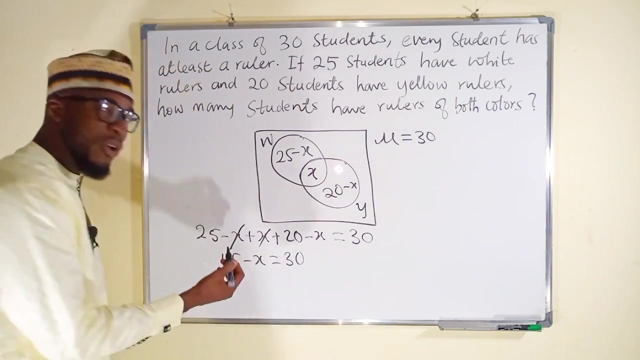 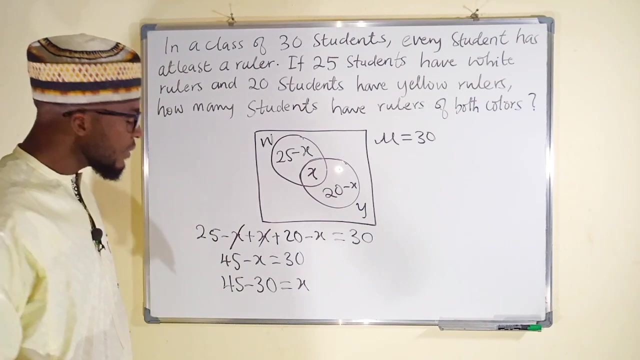 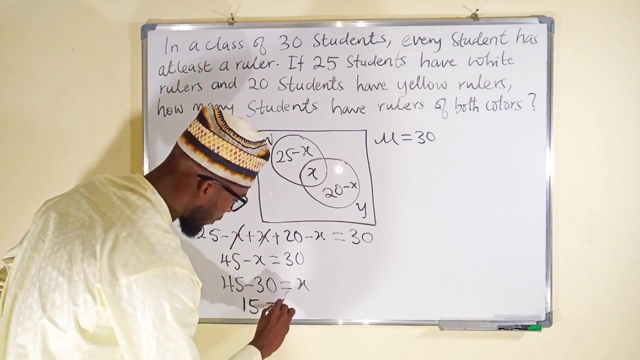 positive. we have: 25 plus 20 is 45 minus X, and that equals 30. we are looking for X, but X is negative here. so we can take it to write so that it becomes positive and bring this one back on. it becomes negative. so we have: 45 minus 30 equals X, and 45 minus 30 is 15. so you can see. 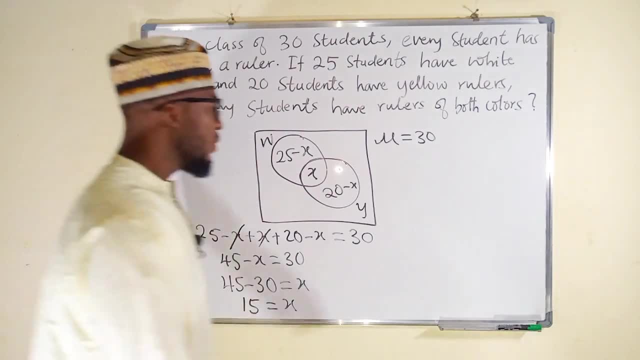 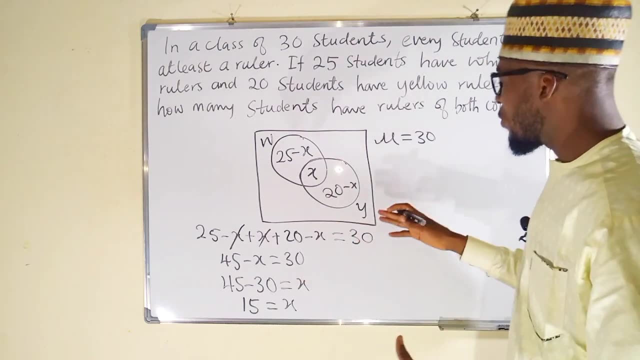 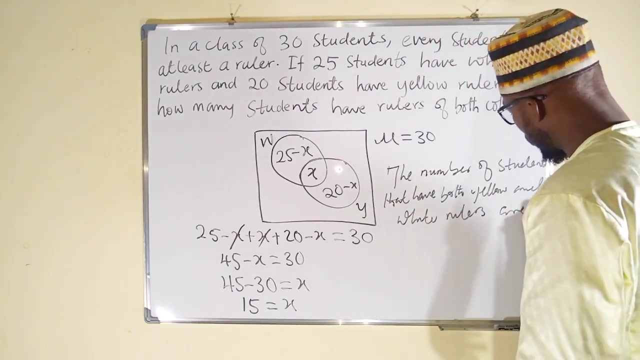 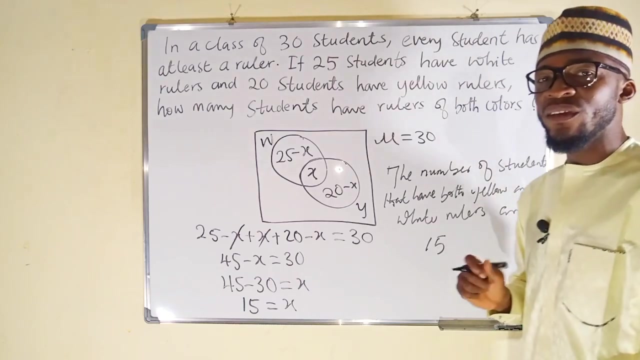 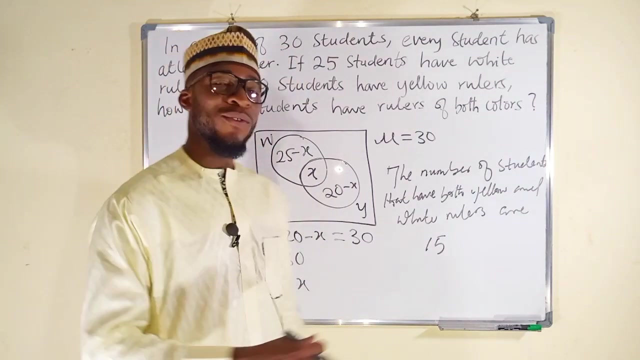 that X is equal to 15. so we we can conclude by saying that the number of students that have both white and yellow rulers are just 15, because X represents them. so you can see it: the number of students that have both yellow and white rulers are 15 and the question answered. thank you for watching and this is all I have. 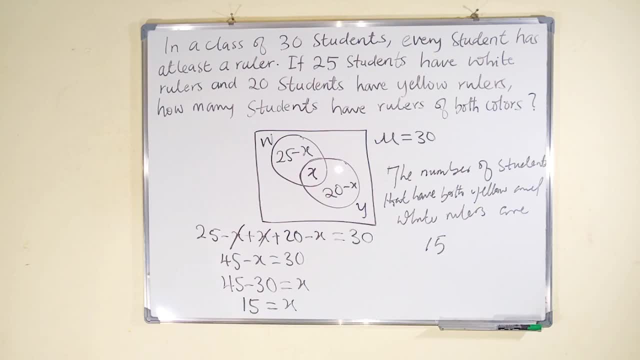 for you today, bye, bye.